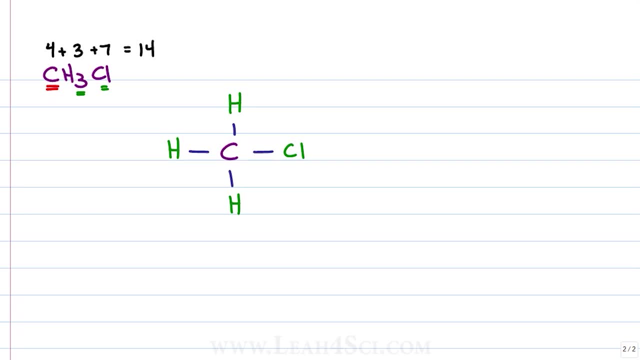 you're going to find. So we're going to take these different numbers. They are the one that have a lot more electrons in them: one, two, three, four around carbon: one, two, three connecting the hydrogen, that's 7. and 8th. one carbon to chlorine, 9,, 10,, 11,, 12,. 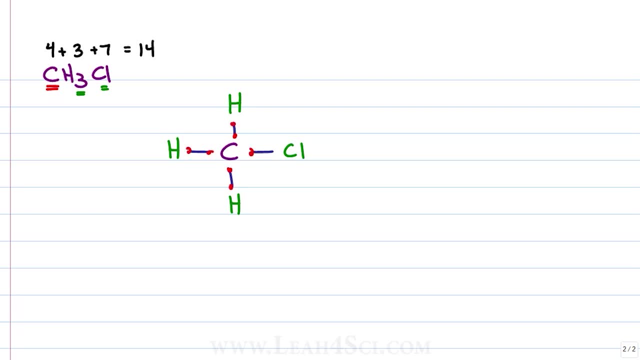 13,, 14.. All of the atoms have a verified complete octet: 8 for carbon and 1 for the nucleic content. 8 for chlorine and hydrogen is an exception where it only needs 2.. We have our Lewis structure. what can we tell about the shape of this molecule? 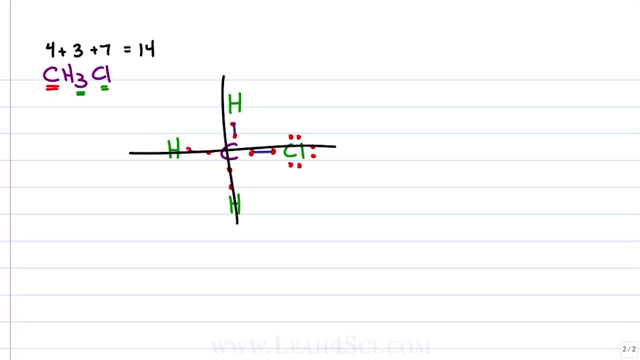 Well, it kind of looks like a flat cross, but it isn't, because the Lewis structure is two dimensional and this molecule is three dimensional. Anytime you have a central atom with 4 groups attached to it, you should recognize that the hybridization for this is sp3 having 4 groups, which means that the molecule is 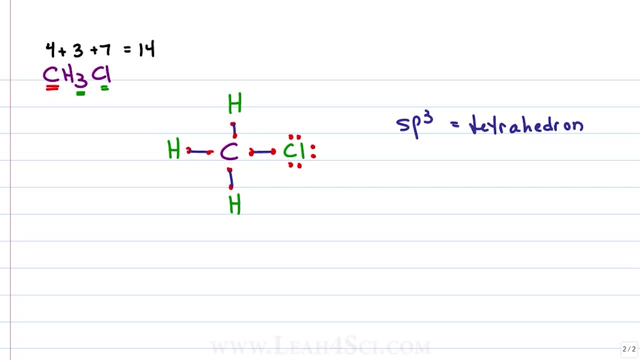 a tetrahedron or tetrahedral? What about polarity? Carbon and hydrogen have a non-polar bond. Carbon and chlorine have enough of a difference in electronegativity, where the electronegative chlorine is pulling electrons away from carbon, making carbon partially positive, giving me 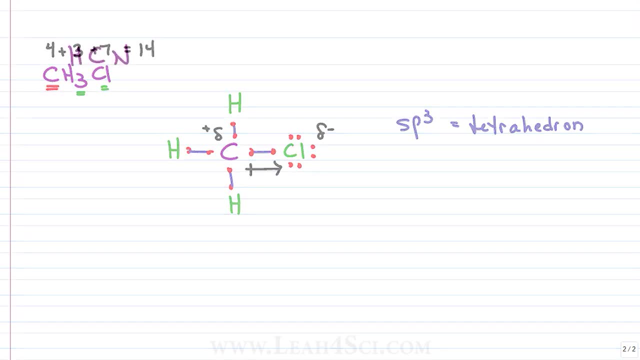 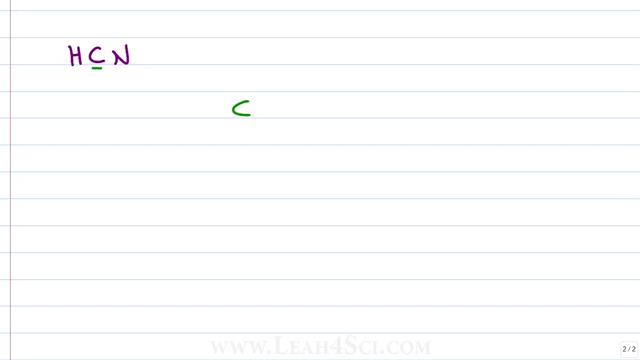 a dipole All in the direction of chlorine. Let's try another problem, looking at HCN For the Lewis structure. let's start with a central atom, which is a carbon, and place the other groups around it. Now we don't have 4 groups to put around carbon, so we'll take what we have put hydrogen on. 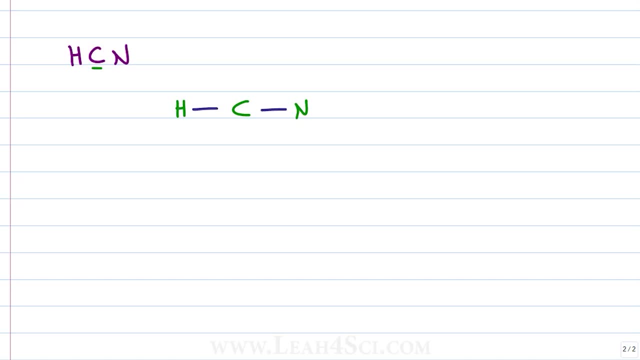 one side, nitrogen on the other, and connect each one with a single bond. How do we know if we're done? We don't until we account for all of the electrons. Hydrogen should have just one valence. Carbon has 4.. 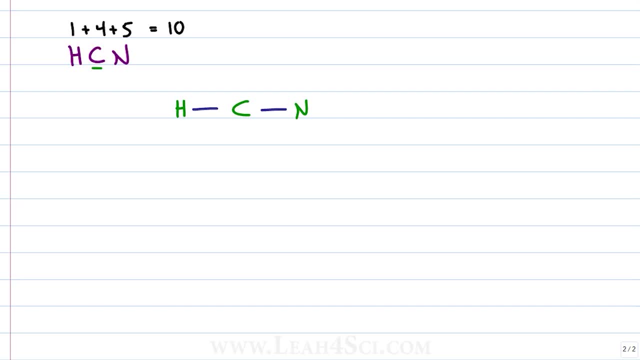 Nitrogen has 5 for a total of 10.. Right now I have 1,, 2,, 3, 4.. That's no good. The question, then, is what to do from here. This is where students get stuck. How do I figure out the number of lone pairs? 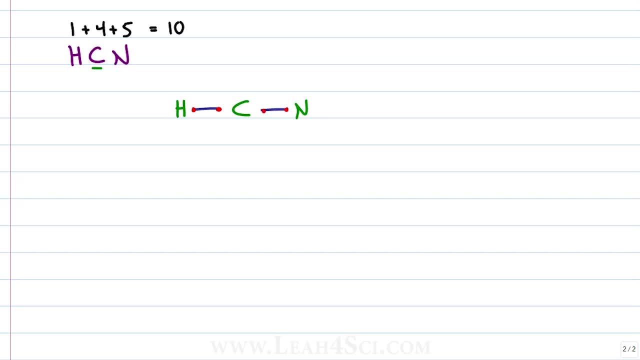 Or maybe pi bonds. The method that I teach in my videos linked below is to first give every atom a complete octet and then compare it to the number of electrons that you should have. If you have too many electrons, We're going to cut out duplicates on neighboring atoms and put pi bonds between them. 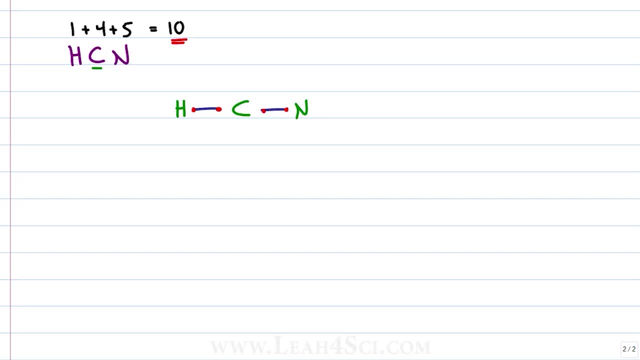 I know this may sound confusing, so if you haven't seen that video, make sure you watch that first. But if you're comfortable with it, let's take a look To complete carbon's octet. we want 8.. So far I have 4,, 5,, 6,, 7, 8.. 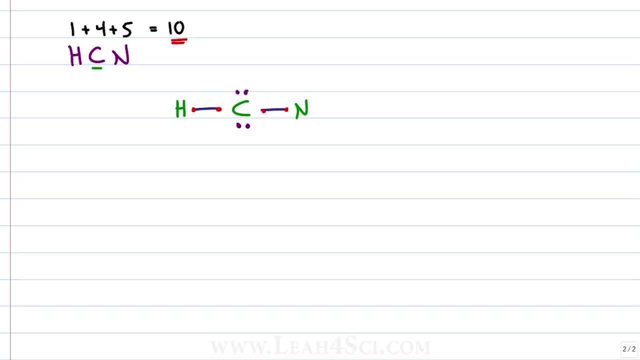 To complete nitrogen's octet. we only have 2. So we have to add 3,, 4,, 5,, 6,, 7, 8.. So we have to add 2,, 3,, 4,, 5,, 6,, 7,, 8.. 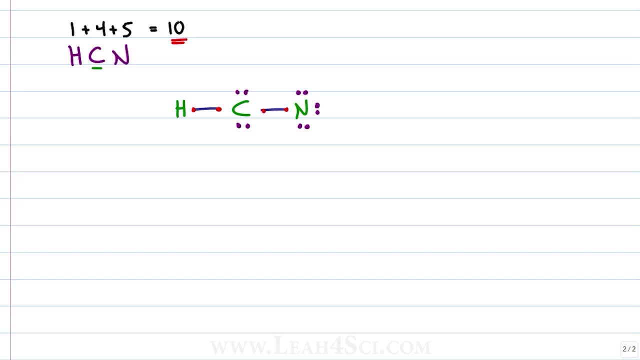 So we have to add 2,, 3,, 4,, 5,, 6,, 7, 8.. But here's the problem: If we count up our electrons, we have 2,, 4,, 6,, 8,, 10,, 12,, 14.. 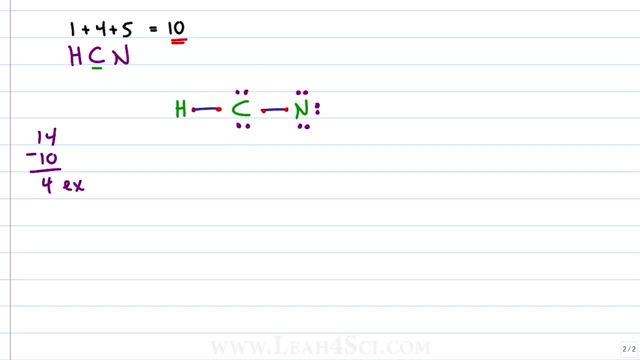 We have 14, we should have 10.. That means we have 4 extra and we have to get rid of it. How do we get rid of 4 extra? We take a pair. we take a pair, that's 4 gone. 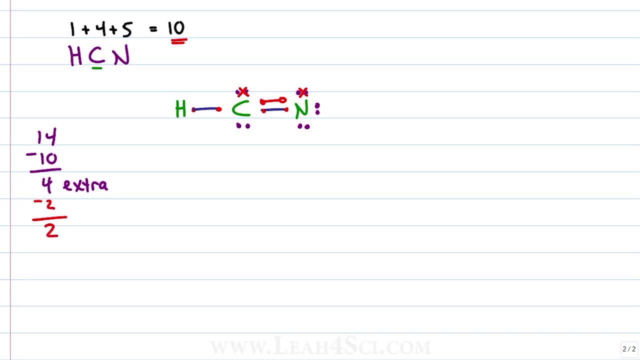 Replace it with a pi bond. We replaced 4 with 2.. We have 2 extra, So we'll do the same thing again over here. Got rid of 4, replaced it with 2 and we have no extras. Let's verify, just to make sure we did it correctly. 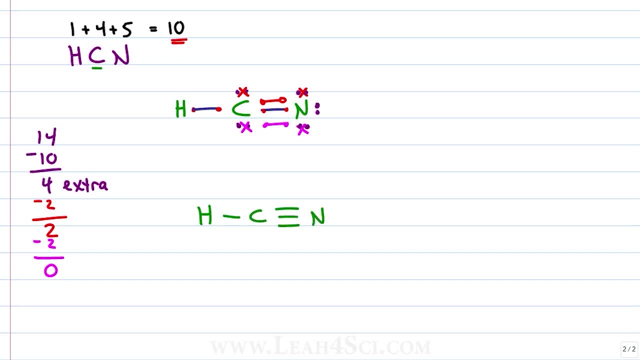 Hydrogen has a single bound to carbon. We give carbon a triple bond to nitrogen and nitrogen has one lone pair on the right side. Let's count our electrons: 1,, 2,, 3,, 4,, 5,, 6,, 7,, 8,, 9, 10.. 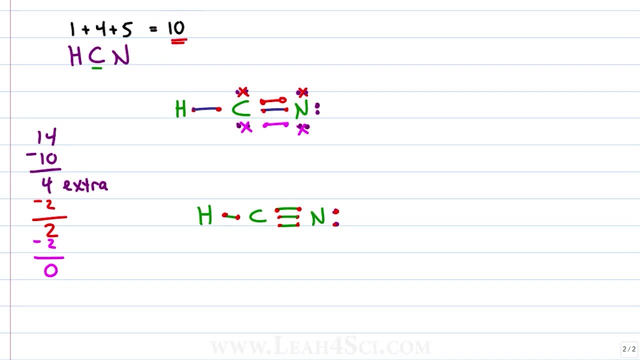 The number of electrons are correct. Does everything have a full octet? Hydrogen has 8.. Carbon has 8.. Hydrogen is an exception to the rule. We have our structure To find the shape of this molecule. we look at that central carbon and it only has two. 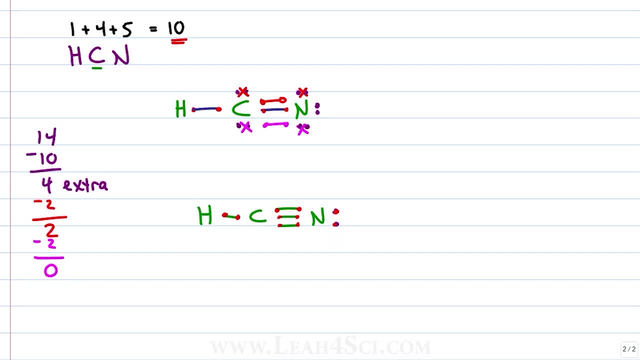 groups coming out of it, One to the right, one to the left, making it a straight line or linear, telling us that the hybridization of that central atom is an sp hybrid. If you're curious, nitrogen is also an sp hybrid because it's got one and two groups. 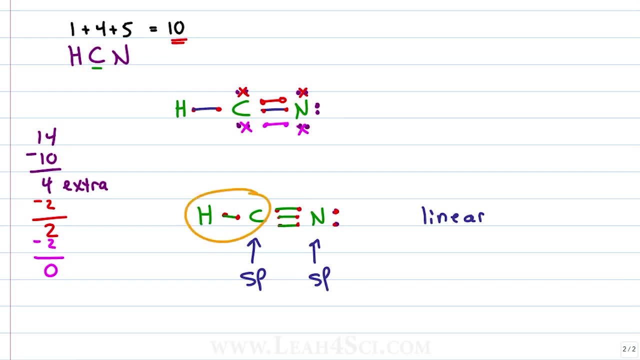 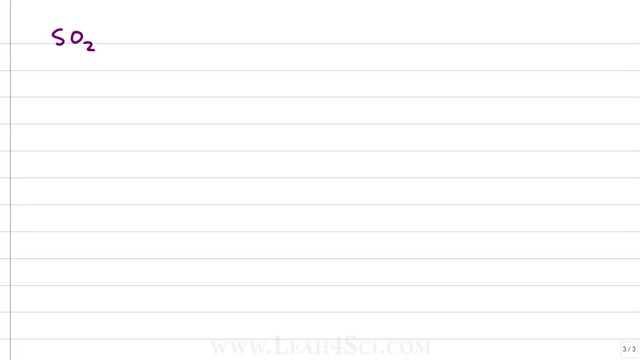 coming out of it. We won't find polarity between carbon and hydrogen, but nitrogen is slightly more electronegative than carbon, and that means it's pulling on the electronegativity, creating a dipole in the direction from carbon to nitrogen. For the next molecule, let's look at SO2, which seems very innocent but can get very confusing. 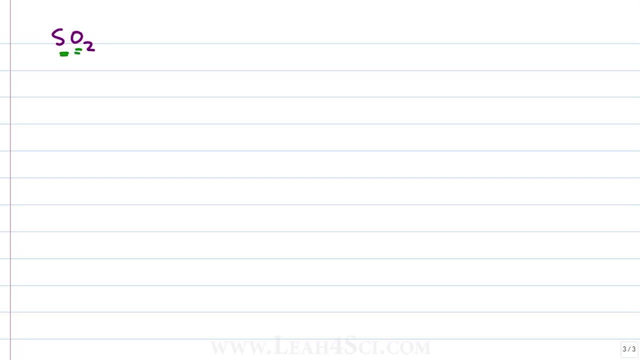 Because we don't have a carbon. do we choose sulfur or oxygen for the central atom? I like to start with carbon. I like to start with a less electronegative atom and put the more electronegative ones around it. So if we have a sulfur, we can put an oxygen on either side and connect them with a single. 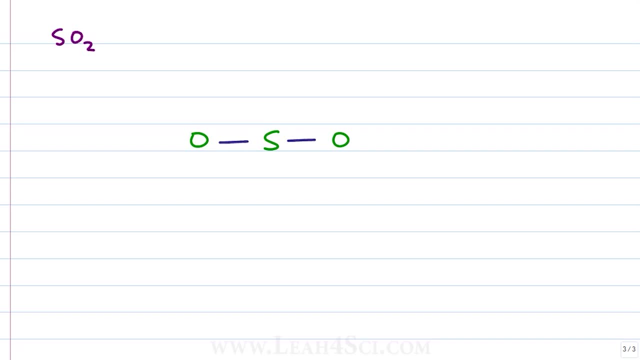 bond. What else do we need for this molecule? Well, how many valence electrons do we have On the periodic table? sulfur is under oxygen, so they have the same number of valence electrons and that means, if each is six times three- one sulfur and two oxygen- we expect a total. 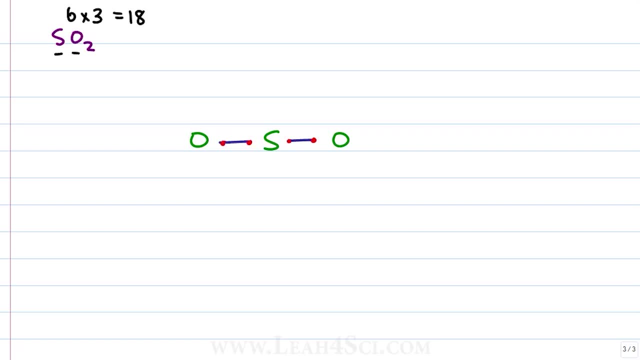 of 18 electrons And so far all I have is four. Let's start by completing all the octets and comparing what we have. A quick count tells us that we have 2, 4,, 6,, 8, 10,, 12,, 14,, 16,, 18, 20.. 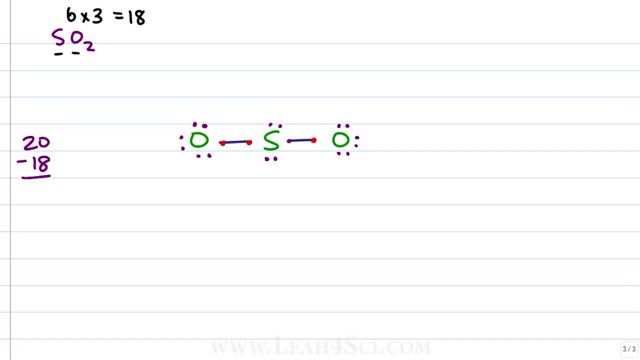 We have 20 electrons. We only won 18.. That means we have two extra that we're going to get rid of by creating a pi bond. We get rid of a lone pair, each on sulfur and oxygen, And put a pi bond between them. 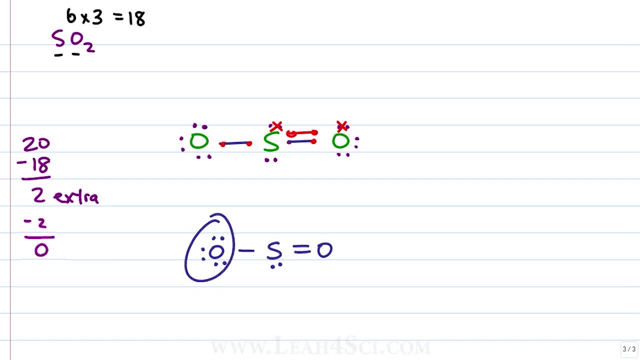 To redraw it cleanly, we see an oxygen with three lone pairs bound to a sulfur with one lone pair double bound to an oxygen with two lone pairs. To find the shape of this molecule we can't simply say it's linear, with sulfur having one group to the right and one group to the left. 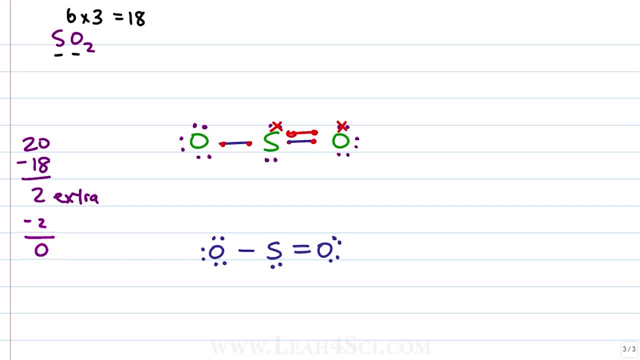 Because that lone pair also counts as a group impacting the shape of the molecule. So, to draw it more correctly, we would have the lone pair on sulfur Taking up a lot of space, forcing the oxygen to shift upward a little bit, Forcing that other oxygen to also shift up a little bit. 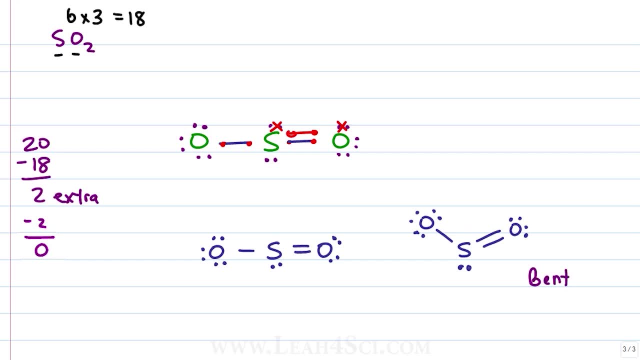 Giving me a molecular shape of bent. Now if you were thinking, wait a minute, if I have three groups, it should be trigonal planar. That would be correct if there was an atom bound here. Having three bound groups gives you trigonal planar. 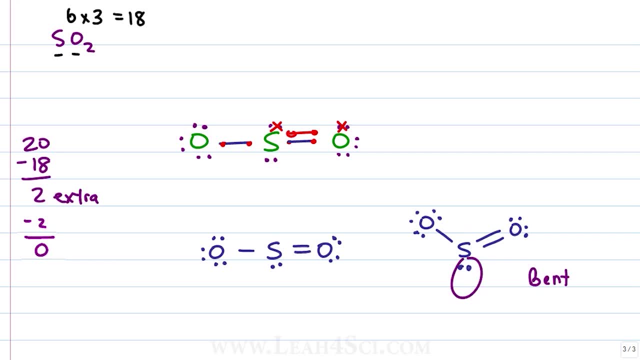 Having only two bound groups, where the third one is a lone pair, Gives you a bent molecule And the hybridization for the central atom- just like something that's trigonal planar- is going to be sp2 hybridized. If you've already studied resonance and formal charge, tutorials for both are linked below. 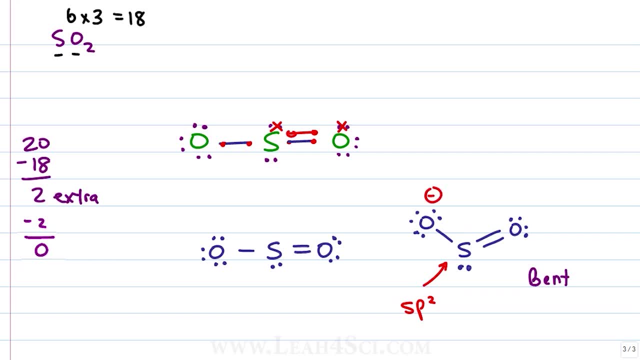 Then you'll recognize that there's a formal charge of minus one on the oxygen and a formal charge of plus one on sulfur, Which would make you realize that we have an unconventional resonance structure where that central sulfur atom can have two bonds. And that's what we're looking for. 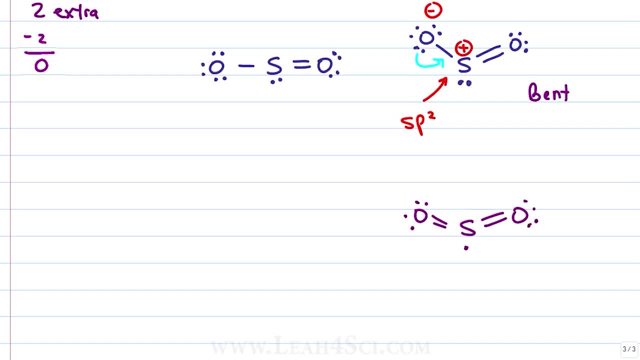 Two oxygens, both double bound and still have a lone pair. If you're thinking, wait a minute, Leia, doesn't this violate the octet rule? Sulfur now has 1,, 2,, 3,, 4,, 5,, 6,, 7,, 8,, 9, 10.. 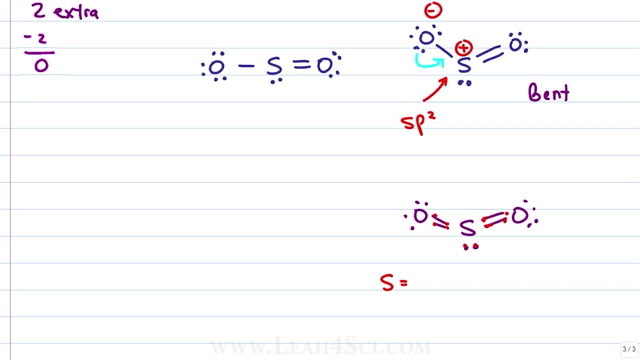 You would be right to think so, except that sulfur is an exception to the octet rule and it can have more than a total of eight electrons in its outermost shell. What about polarity? Given that sulfur and oxygen are somewhat close, What about polarity? 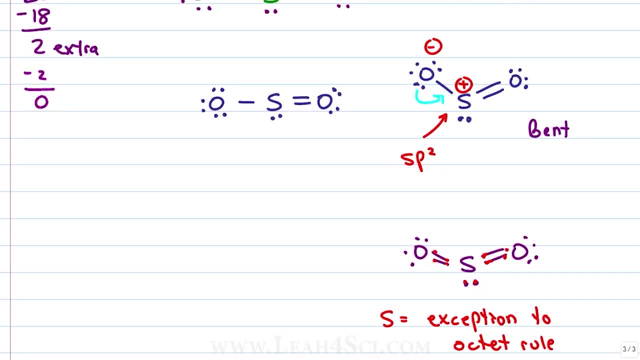 Given that sulfur and oxygen are somewhat close in electronegativity, we wouldn't expect much polarity, but sulfur is still slightly more positive, Oxygen is slightly more negative And in this situation they appear to cancel out, which is why it's important to recognize 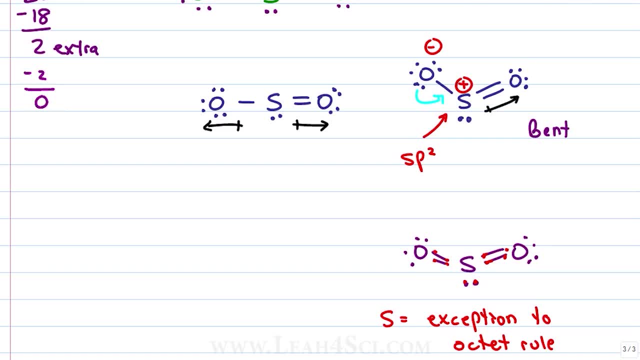 that we have a bent structure where, even though the oxygens are each pulling electronegativity away from sulfur, both of them are pulling in the slightly upward direction, Okay, Which means that the net dipole on this molecule will be canceled out from the right and left. 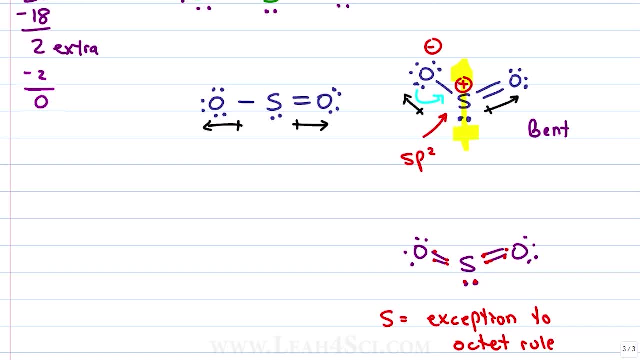 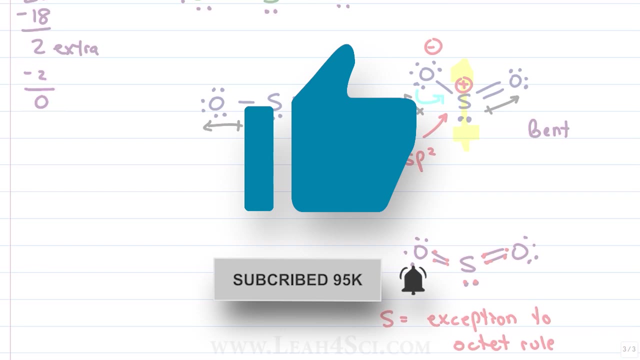 but will go slightly upward, away from sulfur, towards the oxygen. Are you ready to try even more practice? First, make sure to give this video a thumbs up and subscribe to my channel so you don't miss out on any new videos, and then, if you're looking for even more practice, check out.